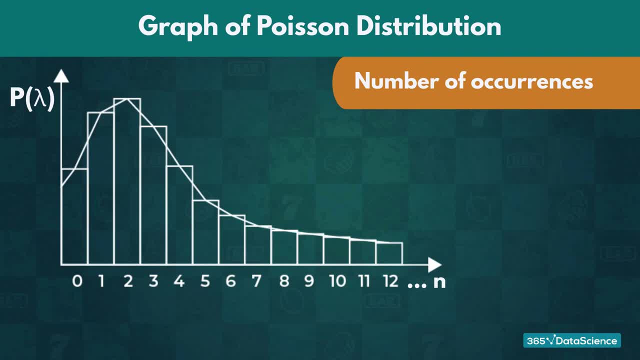 a standard interval of time and the probability for each one. Thus, our graph would always start from zero, since no event can happen a negative amount of times. However, there is no cap to the amount of times it could occur over the time interval. 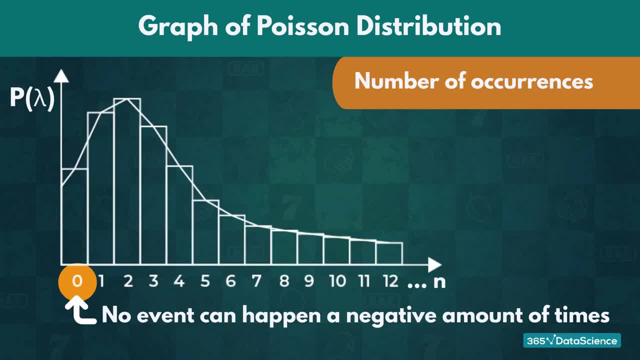 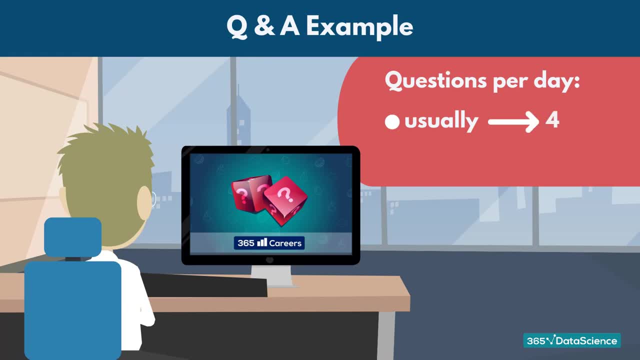 Ok, let us explore an example. Imagine you created an online course on probability. Usually, your students asked you around 4 questions per day, but yesterday they asked 7.. Surprised by this sudden spike in interest from your students, you wonder how likely. 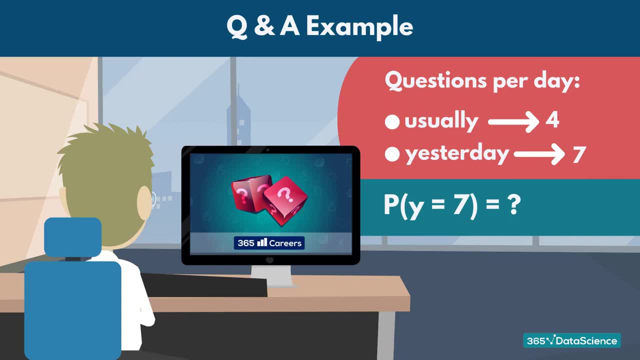 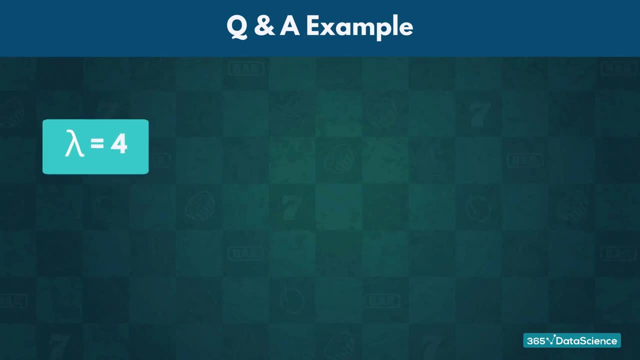 it was that they would ask exactly 7 questions. In this example, the average number of questions you anticipate is 4, so lambda equals 4.. The time interval is one entire workday and the singular instance you are interested in is 7.. 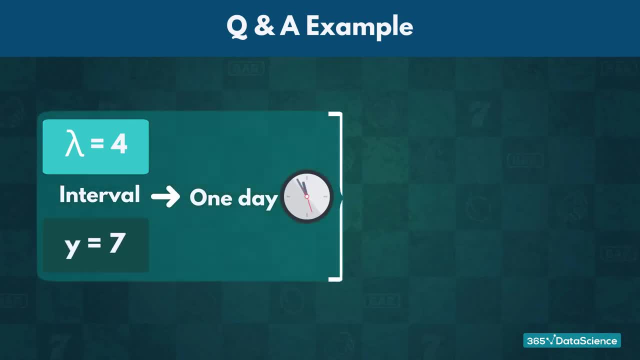 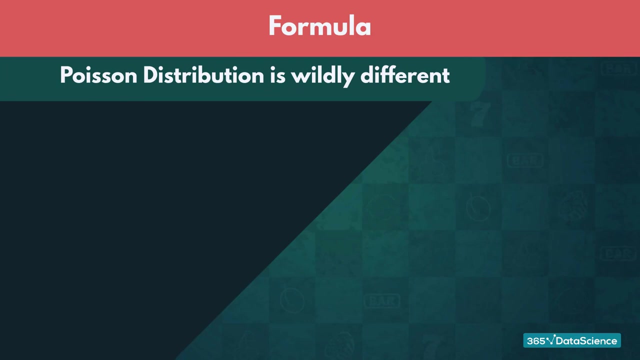 Therefore, y is 7.. To answer this question, we need to explore the probability function for this type of distribution. Alright, As you already saw, the Poisson distribution is wildly different from any other we have gone over so far. It comes without much surprise that its probability function is far different from anything we've 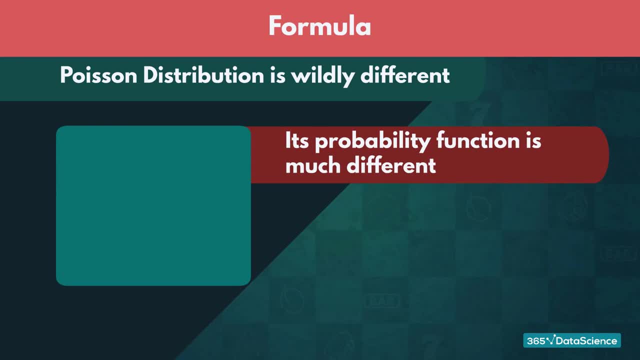 examined so far. The formula looks as follows: P of y equals lambda to the power of y times the Euler's number to the power of negative lambda over y factorial. Before we plug in the values for our course creation example, we need to make sure that 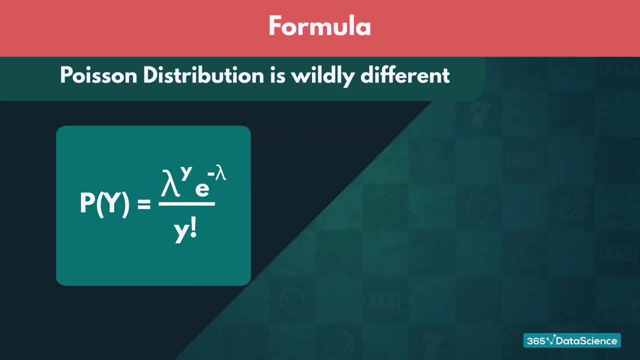 you understand the entire formula. Let's refresh your knowledge of the various parts of the formula. First, the E you see on your screen is known as Euler's number. Euler's number or Napier's constant, as the second name suggests, is a fixed value. 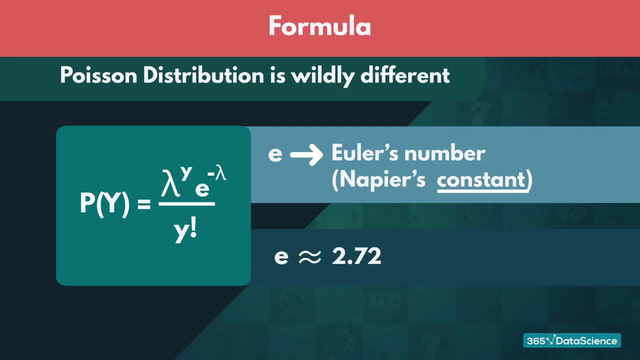 approximately equal to 2.72.. We commonly observe it in physics, mathematics and nature, But for the purpose of this example you only need to know its value. Secondly, a number to the power of negative n is the same as dividing 1 by that number.